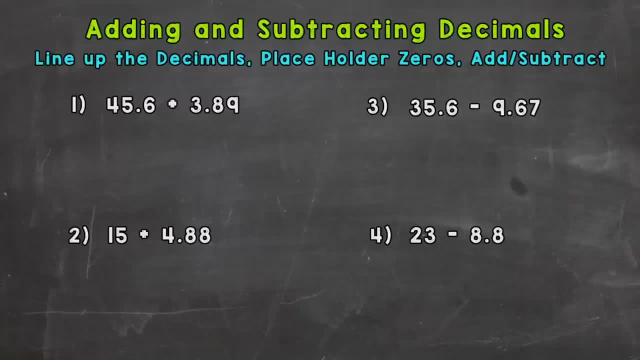 press play when you're ready and check your work with mine. At the top of your screen in blue you see the steps to adding and subtracting decimals so keep those in mind as we work through. 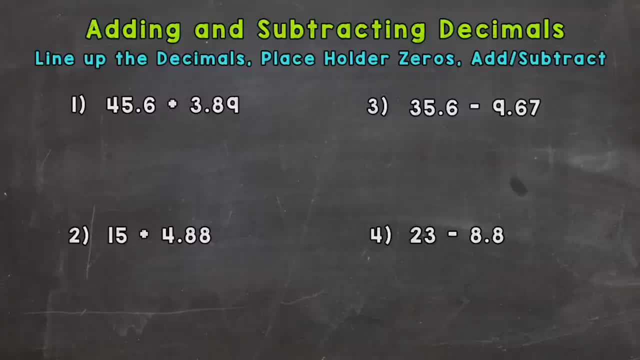 So let's jump right in to number one. So for number one we have 45 and six tenths plus three and eighty nine hundredths. So our first step we need to set the problem up rewrite it vertically or up and down and we need to line up the decimals. So we'll write out 45 and six tenths plus three and eighty nine hundredths. 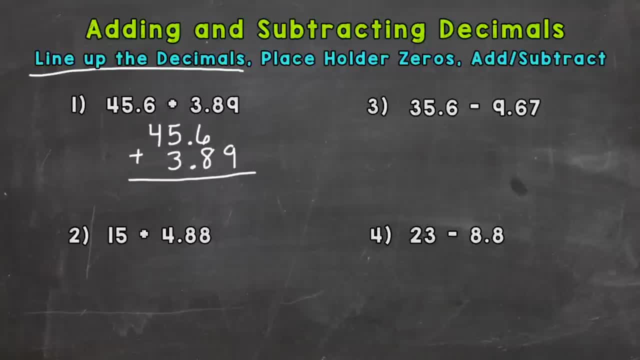 The decimals are lined up therefore all the places are lined up. 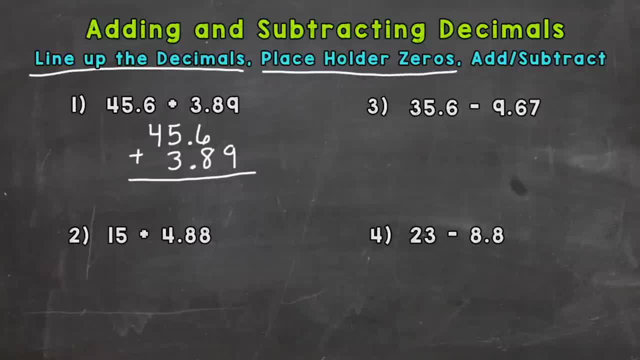 Now we can insert placeholder zeros if need be. So take a look at the nine it's kind of hanging off to the right the three and eighty nine hundredths goes to the hundredths place so we want the 45 and six tenths to go to the hundredths place too. That way we have something above the nine there and it lines up a little better. You can add zeros to the right of a decimal and it does not change the value of that number. So again you can use placeholder zeros to the right of a decimal and it doesn't change the value. This only works for decimals though you can't add zeros to the right of whole numbers or else it does change the value. So use placeholder zeros and then we can add or subtract. So zero plus nine is nine six plus eight is fourteen carry the one bring your decimal straight down. It should be lined up and the decimal will be on the right side of the decimal. 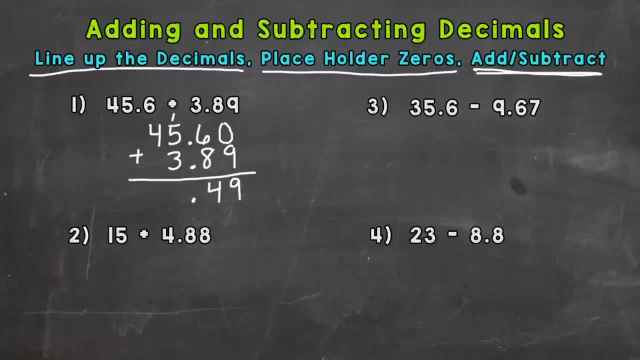 up throughout the whole problem. 1 plus 5 is 6, plus 3 is 9, and then 4. So 49 and 49 hundredths. 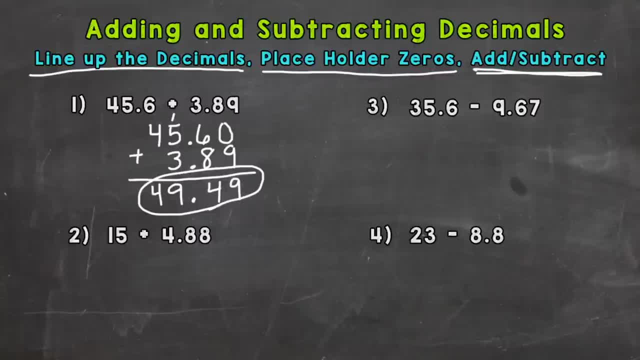 Number 2, we have 15 plus 4 and 88 hundredths. So for a whole number, we put the decimal right after it. Now we can line up 4 and 88 hundredths. And this is addition. So here, the problems offset. Like number 1, we had to use placeholder zeros. So for the 15, we could put a 0 in the tenths and a 0 in the hundredths. Now we're all lined up and ready to add. 0 plus 8 is 8. 0 plus 8 is 8. Bring the decimal straight. Down. 5 plus 4 is 9. 1 plus 0 there is 19. Or I'm sorry, you have the 1 there, which gives us 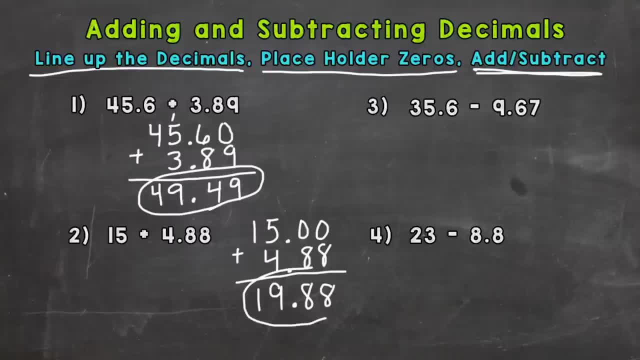 19. So 19 and 88 hundredths. So number 3, we have subtraction, which it's the exact same rules, except when you get to this third step over here, you subtract. So let's write out our problem, lining up the decimal. 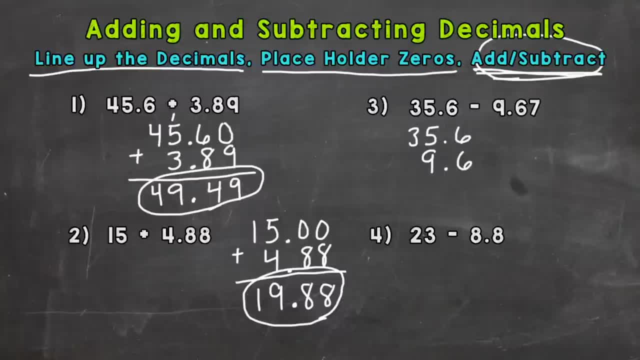 And it's subtraction. So let's put the placeholder 0 there. And now it's time to subtract. So we cannot do 0 minus 7, so we need to borrow. So now we have 10 minus 7, which is 3. Cannot do 5 minus 6, so we need to borrow. So we get to 15 minus 6, which is 9. Bring the decimal straight down. So we need to borrow again. We can't do 4 minus 9. So we need to borrow from the 3 or the tenths place here. And we get 14 minus 9, which is 5. And then we have the 2. So 25 and 93 hundredths. Line up the decimals. Use placeholder 0s. Add or subtract. But just like number 2 here, we have a whole number in number 4. So the 23. And we put the decimal right after. Then we have 8 and 8 tenths. And subtract. So let's put the placeholder 0. And we are ready to solve. So we can't do 0 minus 8. Don't just drop the 8 there. We need to borrow.